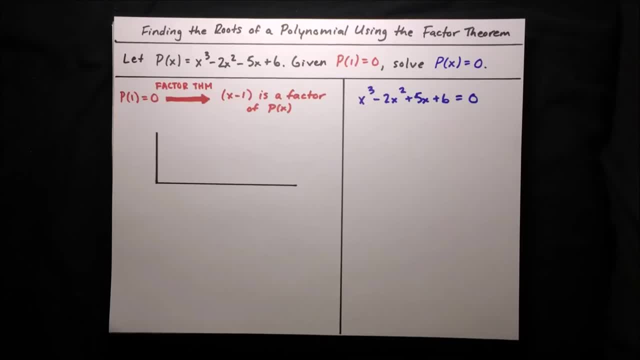 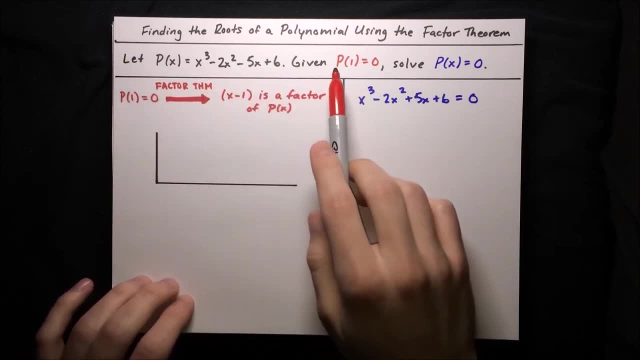 In this video I'm going to show you how to find the roots of a polynomial using the factor theorem. So we've got a polynomial, x cubed minus 2x squared, minus 5x plus 6, and we're given that p of 1 equals 0 and we want to solve the 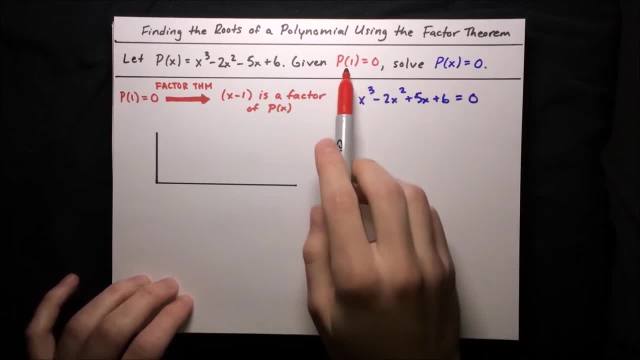 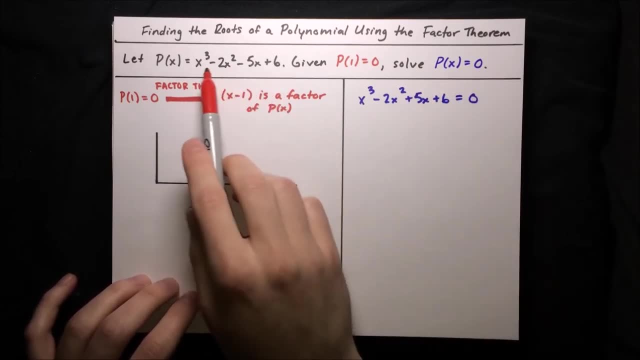 equation: p of x equals 0.. So really, we're given that 1 is a root of the polynomial and we want to find the other roots. Okay, so p of x equals 0. if we substitute in the expression for the polynomial, that just becomes the polynomial, the x cubed. 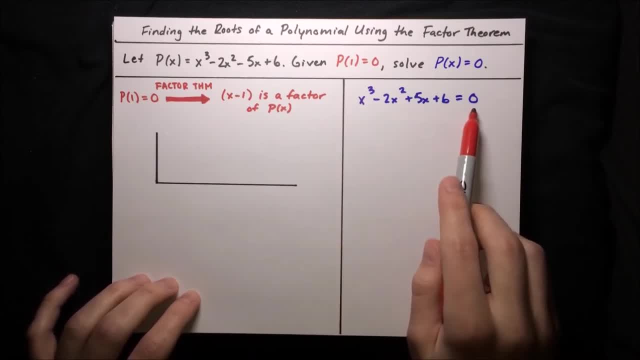 minus 2x, squared plus 5x with 6, that is equal to 0, and in order to solve this equation, we'd ideally like to factor this polynomial, so that way we can just use the 0 product property and set each factor equal to 0, which is a. 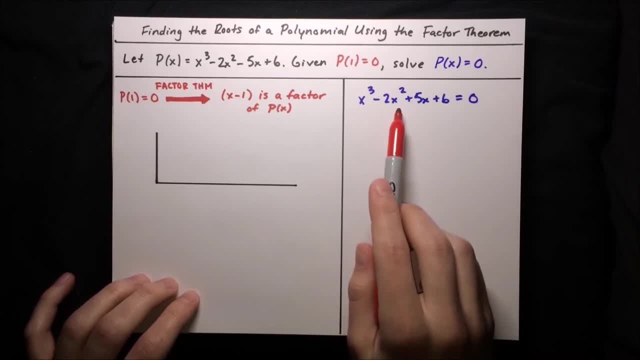 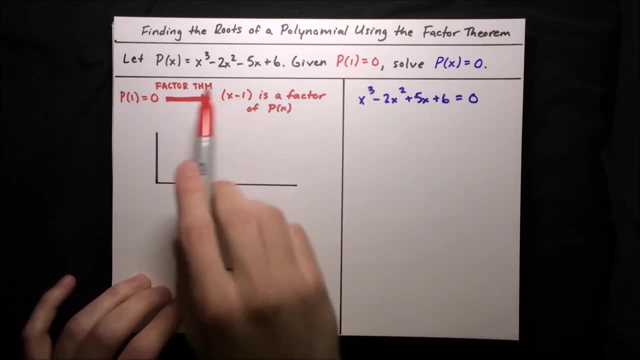 lot easier to solve, but factoring, of factoring a cubic, is pretty tricky. so how are we going to do this? well, well, thankfully we have that p of 1 equals 0 and, according to the factor theorem, since 1 is a root of the polynomial x, 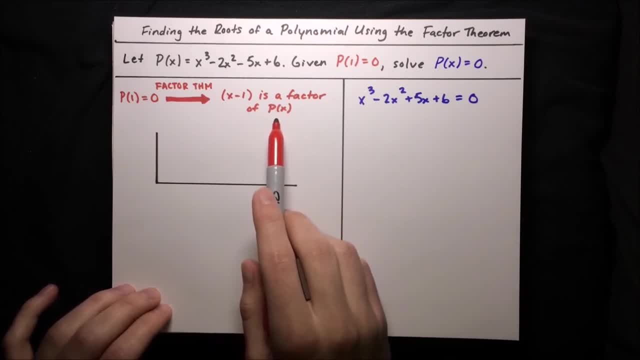 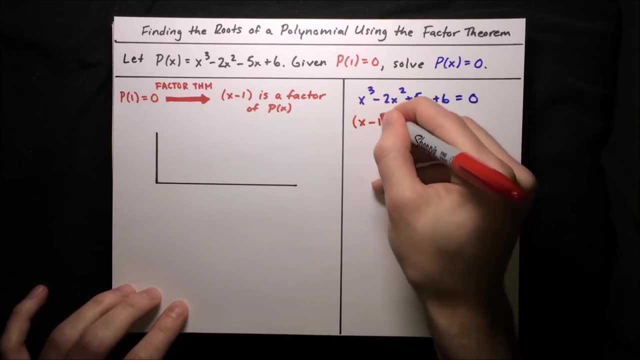 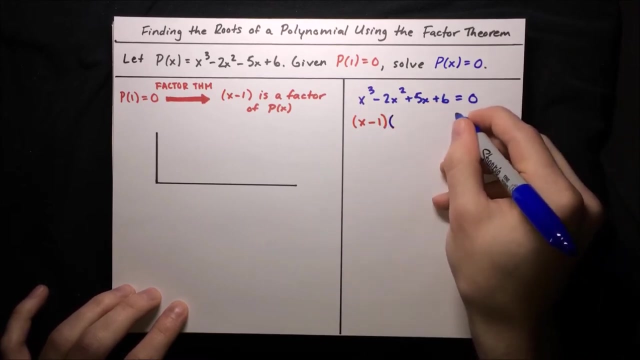 minus 1 is a factor of the polynomial. so that means we already know one of the factors, so why don't we write this down? so X minus 1 is one of the factors, and now we know that the next factor, whatever X minus 1 multiplies, has to be a quadratic. and 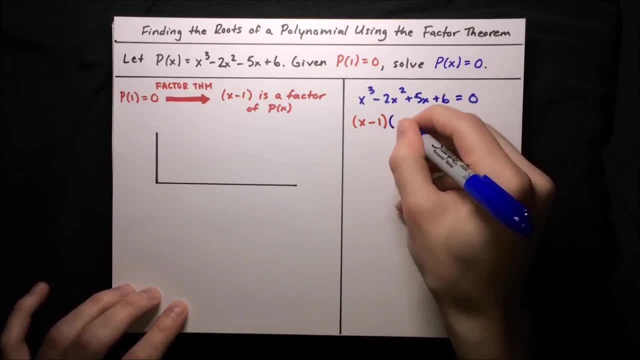 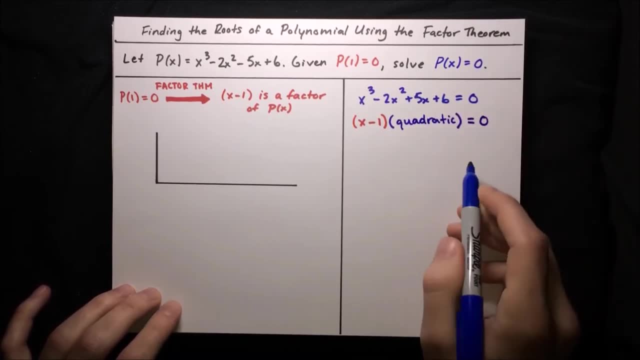 quadratics are a lot easier to solve. so quadratic, we'll just write in quadratic and we'll fill that in in a bit, okay, so quadratics are pretty easy to factor. but first of all, what is the quadratic here that multiplies X minus 1 here? well, in. 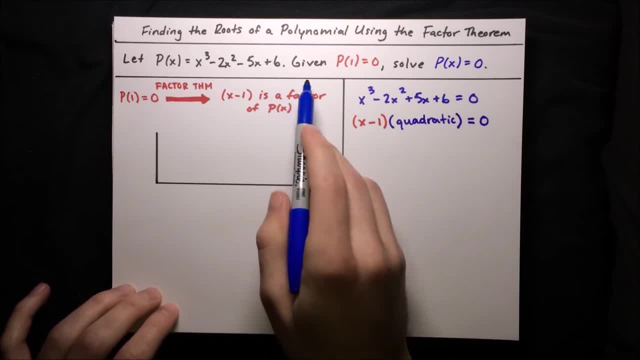 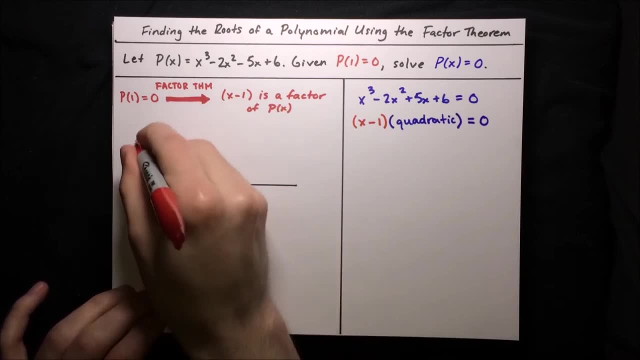 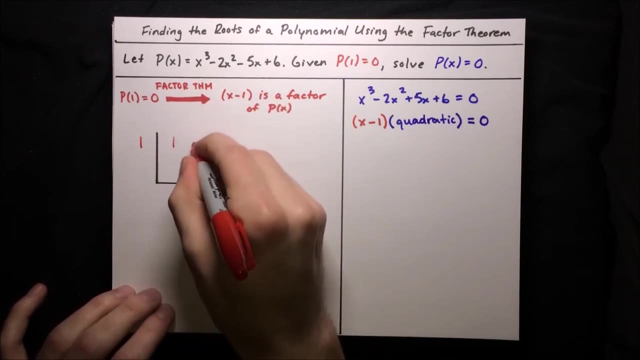 order to find that we can just divide our polynomial by the factor X minus 1, and we can just use synthetic division to do that. so take that root 1 and put that on the left corner here, left top corner, then put the coefficients of P above, so there's 1x cubed, then minus 2x squared, then minus 5x, then plus 6 is our. 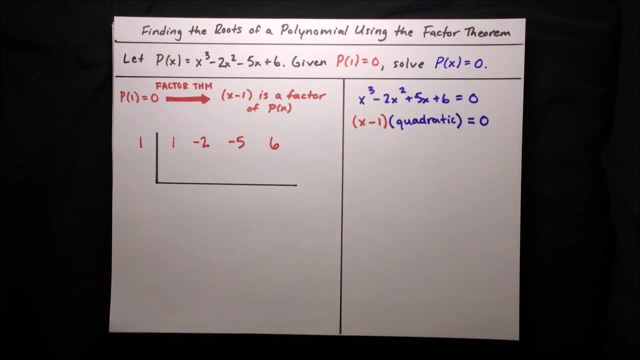 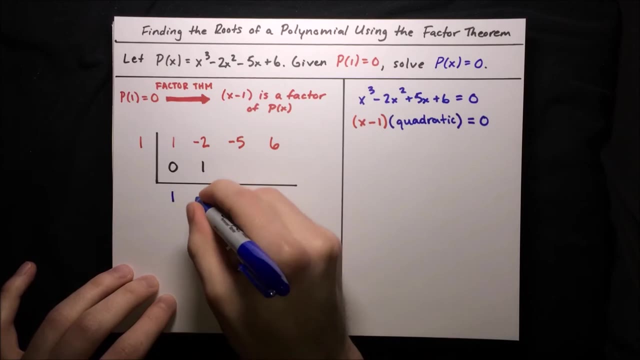 constant, and now we're going to multiply that by the factor X minus 1, so that's Red estaban. then 1x1 is 1, then add down the column negative. 2 plus 1 is negative 1, and then multiply 1 times negative. 1 is negative 1, and then add down the column. 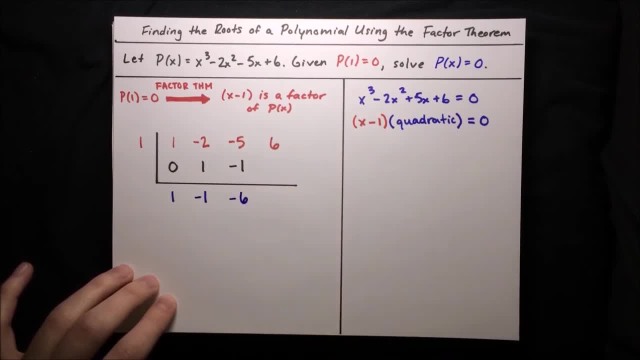 negative 5 Plus negative one is negative, and then multiply 1 to the direito times negative 6 is negative 6, and then add down the column 6 plus negative 6 is just 0.. Okay, so these tell us the coefficients of our quadratic, and the quadratic would just be then 1x squared. 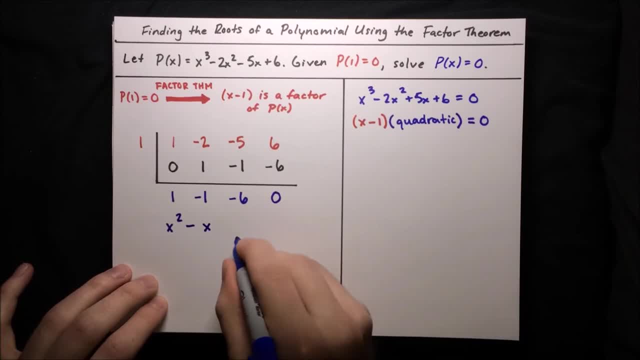 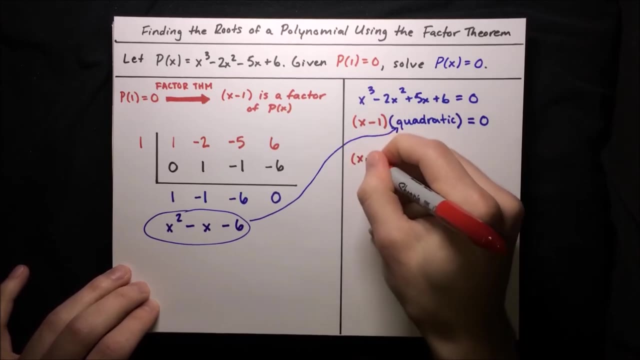 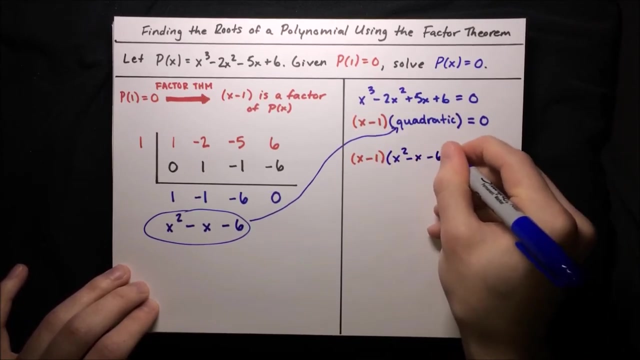 then minus 1x, and then minus 6 and then no remainder. So this here is our quadratic that we're going to put in for there. So let's go ahead and write this down again with the quadratic inside. So x minus 1 times the quadratic x squared minus x minus 6, that has to be equal to 0.. 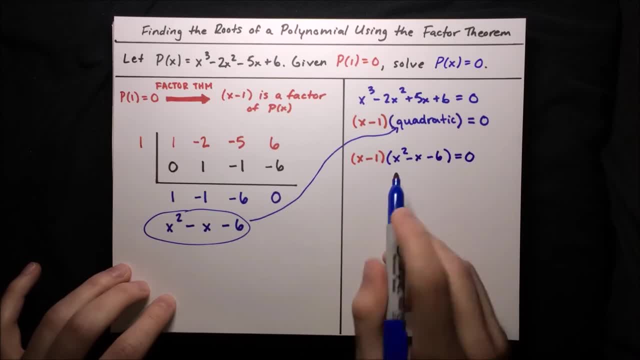 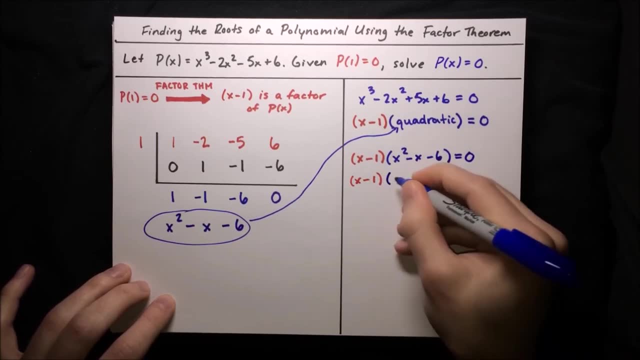 And now let's go ahead and continue factoring this quadratic. So write down the factor x minus 1 first, and then what does this quadratic factor into? Well, there's is an x and x negative 6. that suggests 2 and 3 for factors, because they have to sum to negative 1. 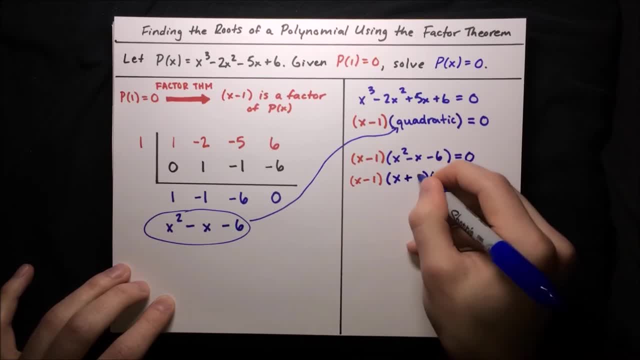 so we'll have a negative 3 and a positive 2. that way, negative 3 plus 2 is negative 1. 2 times negative 3 is 6. good, all checks out, and now let's go ahead and use the zero product property to set each. 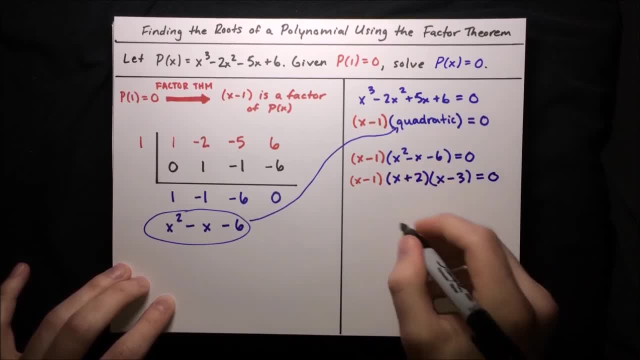 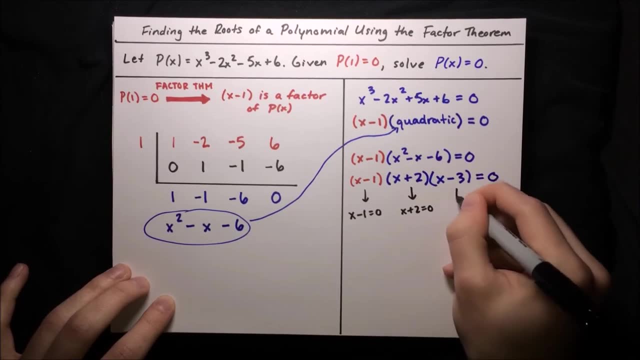 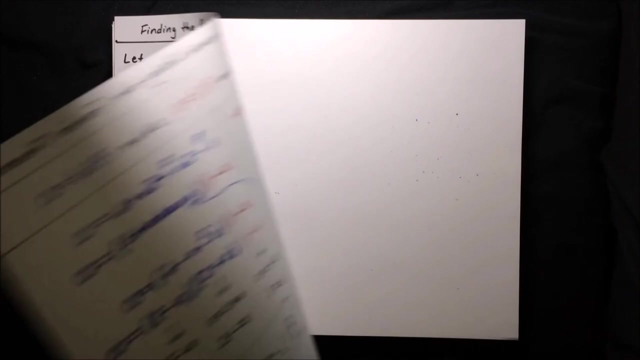 factor equal to zero, so zero product property says that the solutions would then be: x minus 1 equals 0, x plus 2 equals 0, x minus 3 equals 0, and these are all easy to solve: either x equals 1, or x equals negative 2, or x equals 3. so that's our solution: set 1, negative 2 and 3. here's another. 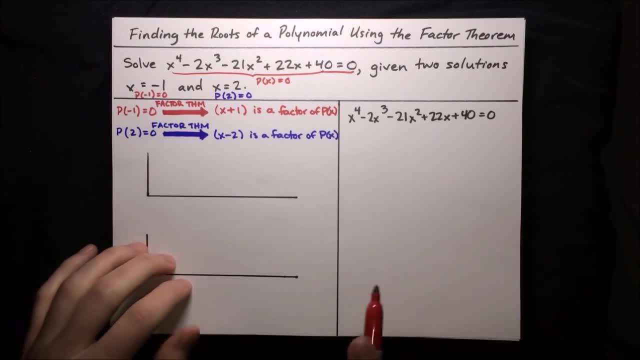 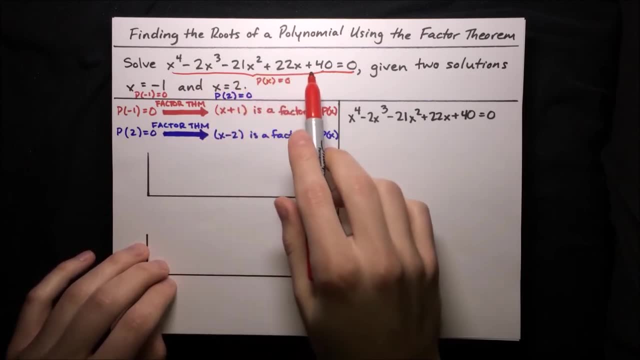 example, which is pretty similar to the previous one. The difference here, though, is that now we have a fourth degree polynomial with x to the fourth. minus 2x, cubed, minus 21, x squared, plus 22x plus 40 equals zero, and we want to solve this equation. 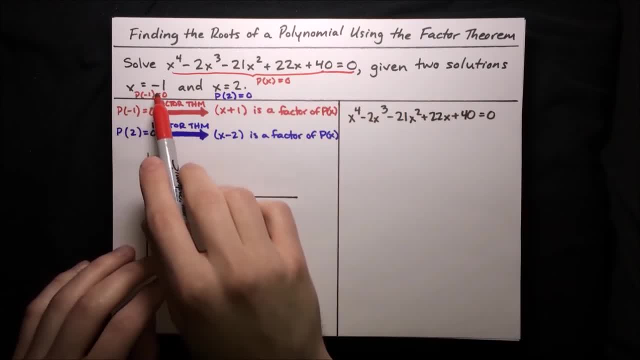 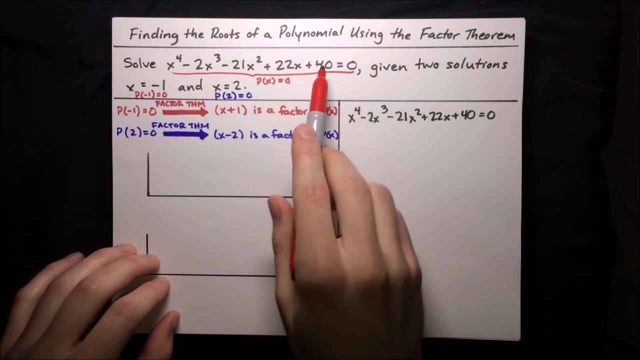 given two solutions of the equation. The solutions are: x equals negative one and x equals two. but we're going to approach this in the same way that we did in the previous problem. We're just going to say: let's let this left hand side here, let's let that be the polynomial p, so that this equation 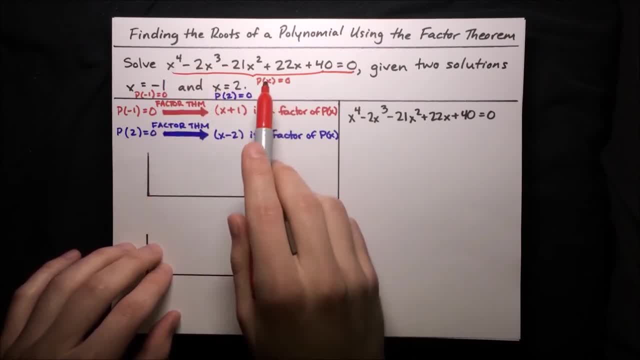 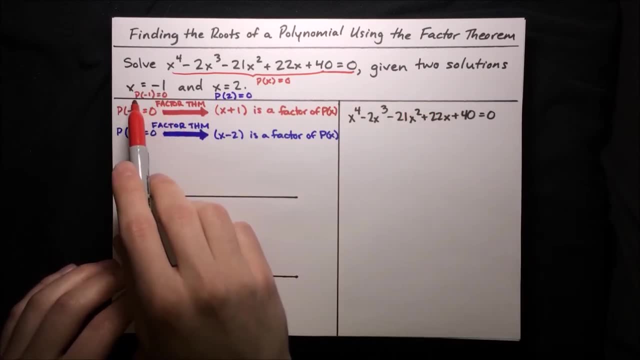 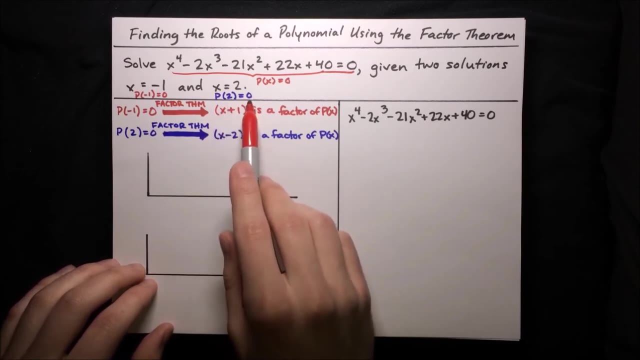 is really just saying that p of x equals zero. We really just want to find the roots of this polynomial and we're given two roots. The solution x equals negative. one corresponds to a root p negative one equals zero. and solution x equals two corresponds to root two. p of two equals zero. 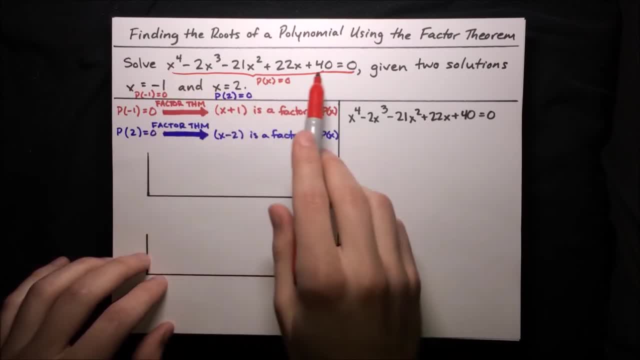 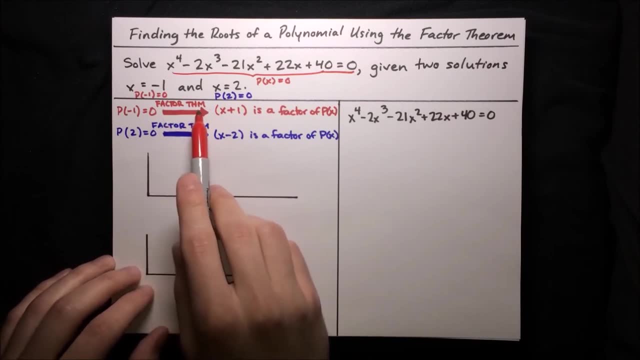 and so we want to factor this fourth degree polynomial and we have two factors according to the factor theorem. Factor theorem tells us that since p of negative one equals zero, then we know that x plus one is a factor of p of x. remember you just flip the sign. 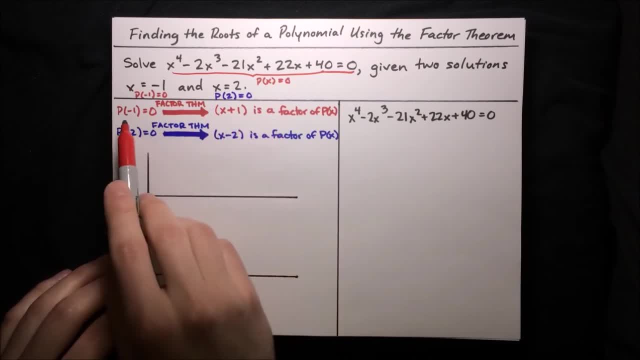 on on the root here. to get the factor negative one goes to positive one. it's kind of like x minus negative one, so that turns into x plus one and then p of two equals zero according to the factor theorem. that tells us that x minus two is a factor of p of x. so why don't we use these two? 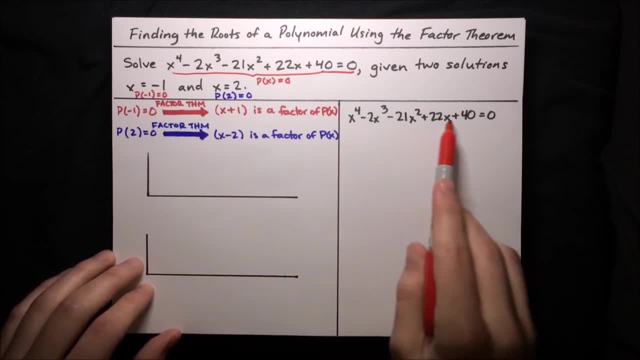 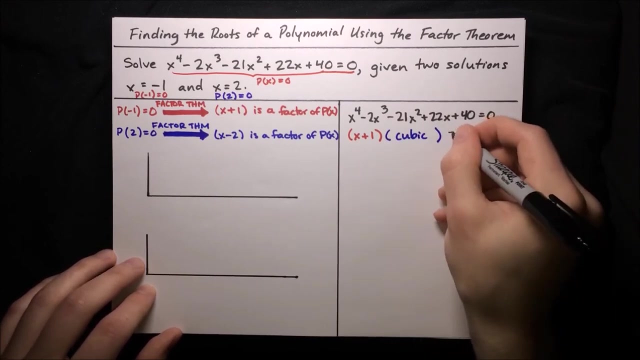 factors to break down this polynomial into more factors using synthetic division. so first of all we're- let's focus on this factor x plus one. so i'll have x plus one here. x plus one will be a factor, and then we'll have another factor which is a cubic, and that's going to all be equal to. 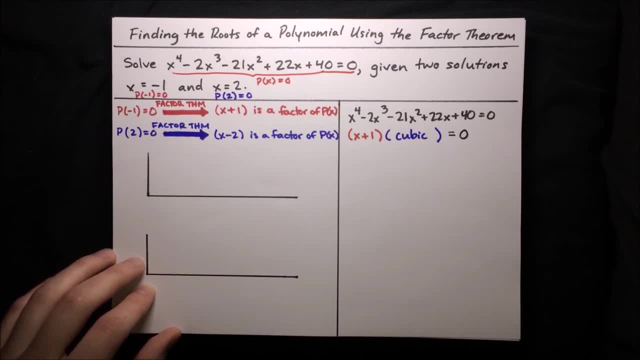 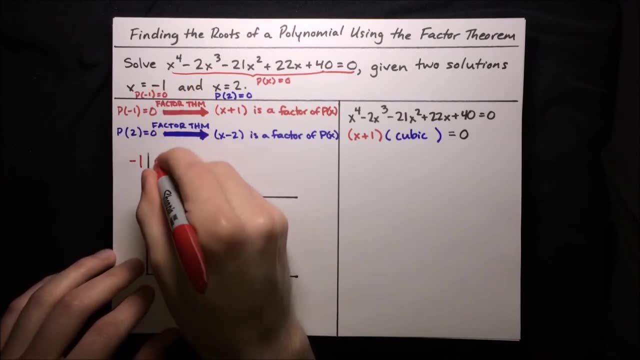 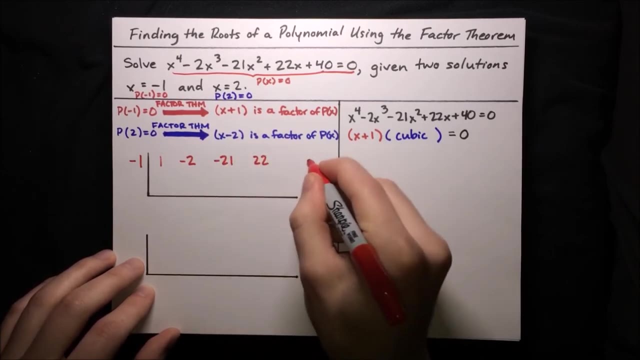 zero. so let's figure out what that cubic is. we can just do that using synthetic division. here you put in the root on the top left negative one, and we'll put in our coefficients: one x to the fourth, then minus two x third, then minus 21 x squared, then plus 22 x, then plus 40.. now let's go ahead. 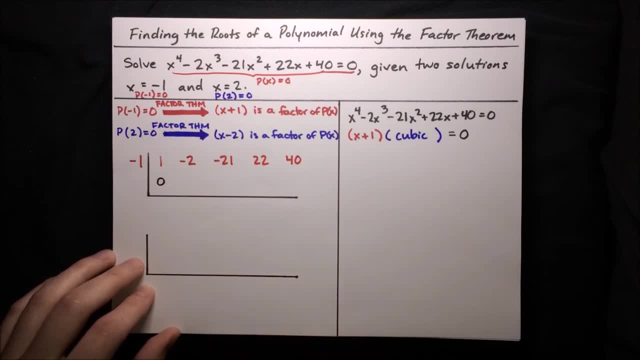 and start it off with a zero here. so adding down the column one plus zero is one, then times negative one, that gives us negative one. then add down the column to get negative three. then multiply by negative one to get positive three. then add down the column to get negative 18. 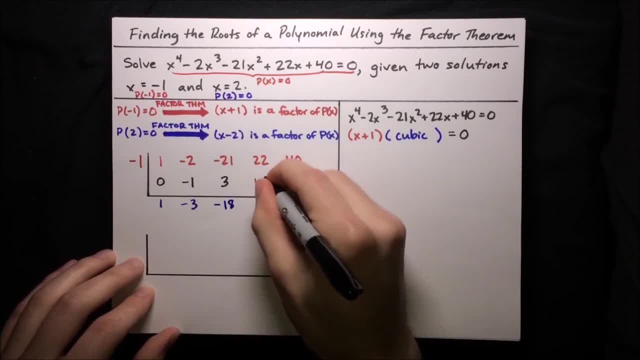 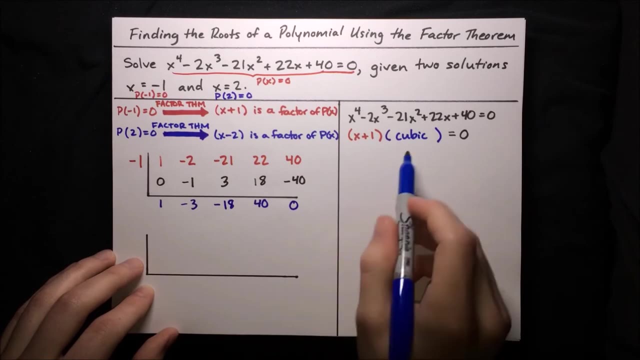 then multiply by negative one to get positive 18, then add down the column to get 40, and multiply by negative one to get negative 40, and then add down the column to get zero. so great. so now this is telling us the coefficients. on our cubic it's just 1x. 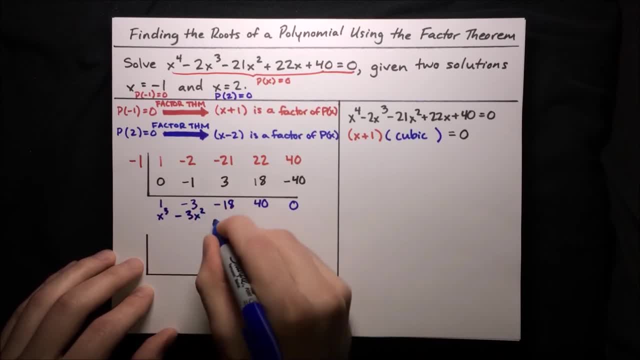 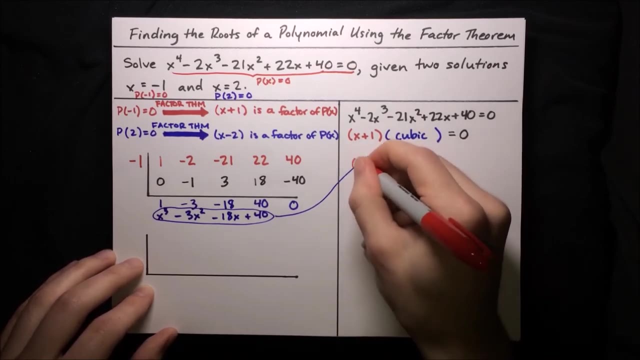 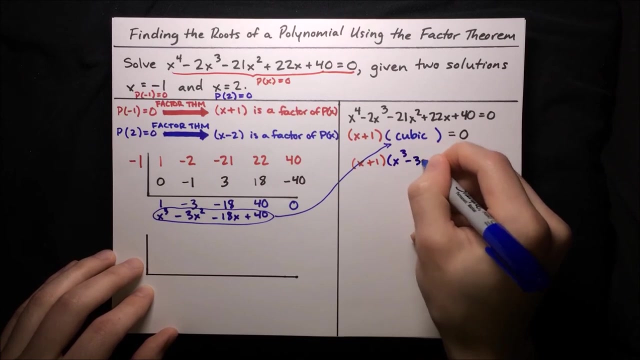 cubed and then minus 3x squared, then minus 18x and then plus 40, so that cubic is going to go in for our cubic there and then we can write the equation again. so this is just x plus 1 times our cubic times, our cubics: x cubed minus 3x. 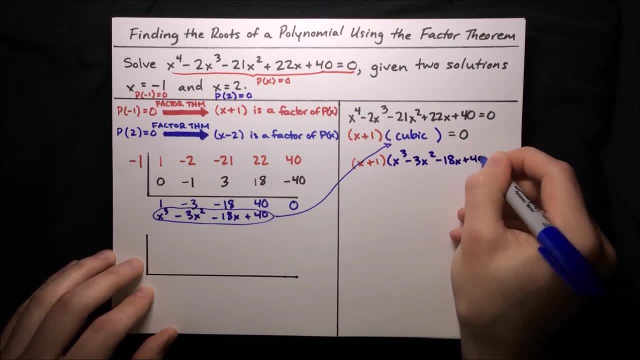 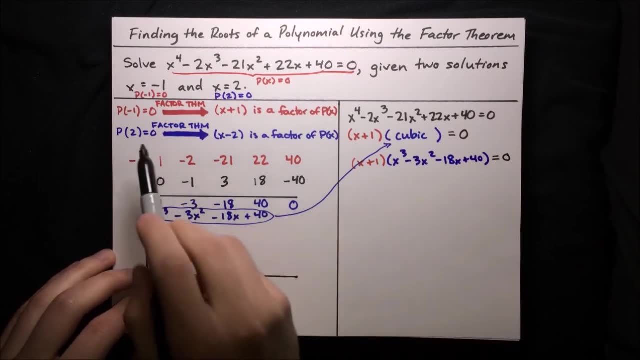 squared minus 18x plus 40, and that has to equal 0. ok, great, great. now let's use our second factor to break down this cubic a bit. so we've got: x plus 1 is a factor. we also know that x minus 2 has to be a factor. 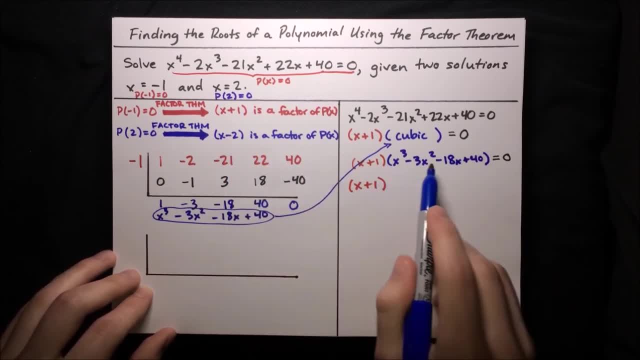 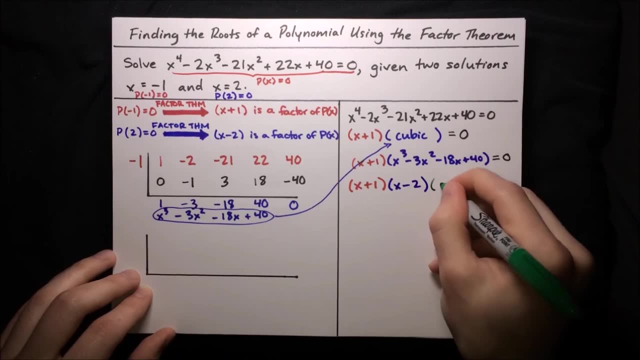 um. so x minus 2 has to be a factor in this cubic here. so we can write this as x minus 2 times some other quadratic expression, and again we can just perform synthetic division to figure out what that quadratic is. so let's go ahead and 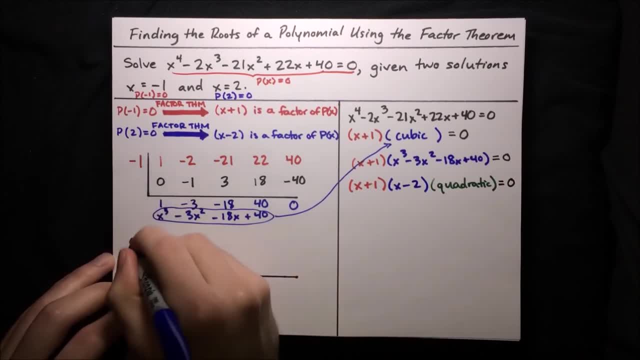 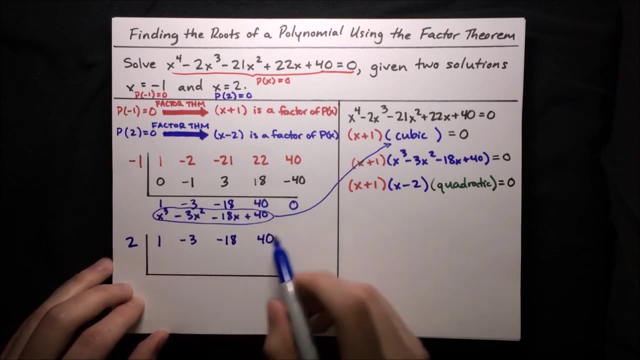 write down our, our root here. root is 2 and we'll write down the coefficients of the cubic, that's 1x cubed, then minus 3x squared, 3x squared minus 18x, then plus 40, and we'll go ahead and perform synthetic division to divide: 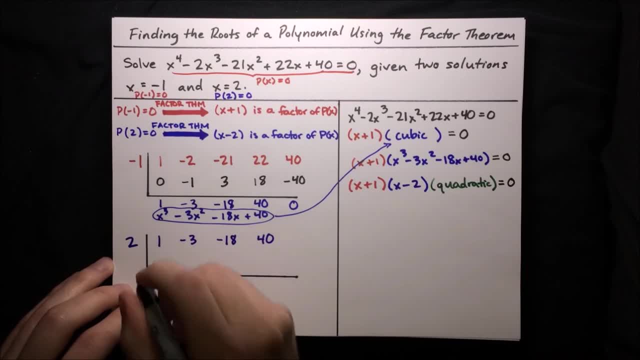 that cubic by this linear factor. Let's see what we get. So start it off with zero. add down the column 1 plus 0 is 1, then multiply 2 times 1 is 2,. add down the column negative 3 plus 2. 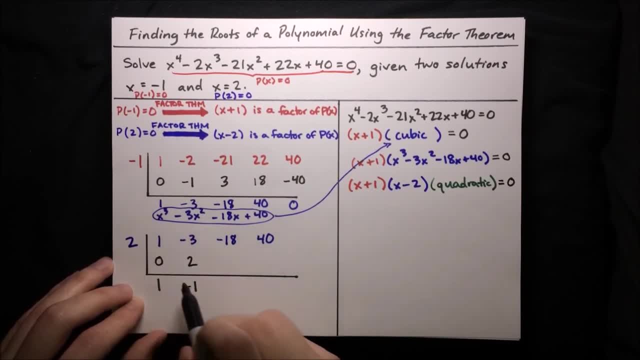 is negative 1, multiply that by 2, you get negative 2, add down the column to get negative 18 minus 2 is negative 20, then multiply that by 2 to get negative 40, and then add down the column and you. 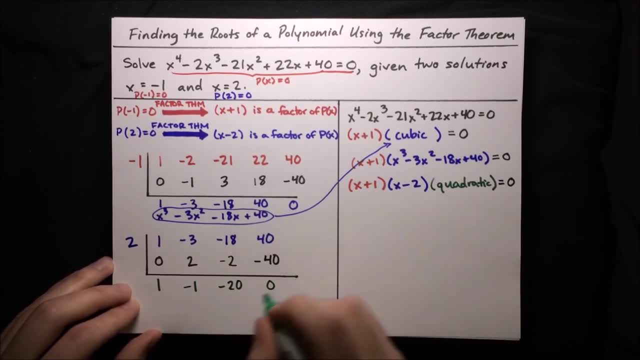 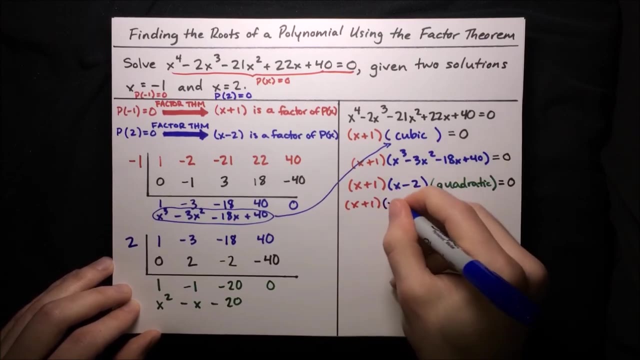 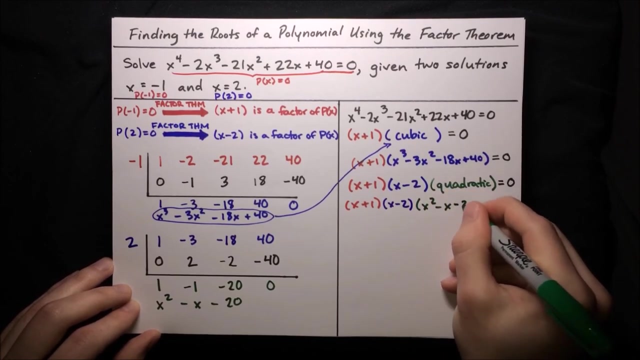 just get zero. So these tell us the coefficients in our quadratic. So just 1x squared, then minus 1x, then minus 20.. Okay, let's put that in, So x plus 1 times x minus 2 and then times our quadratic x squared minus x minus 20.. That has. 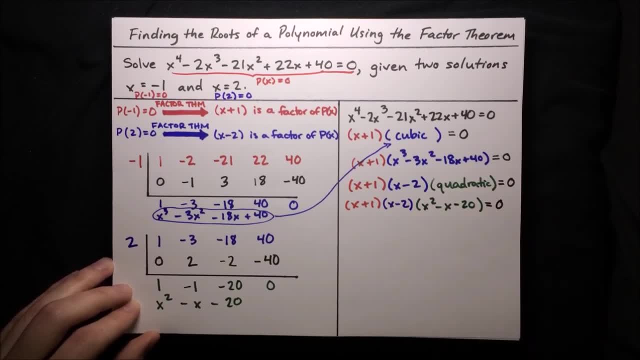 to equal zero and let's see if we can factor the quadratic anymore. Let's write down our two factors here, x plus 1 and then x minus 2, and then looking to factor the quadratic. So this has to multiply to 20. And multiply to negative 20, sum to negative 1.. Well, 5 and 4.. 5 and 4 will work. One of them should be: 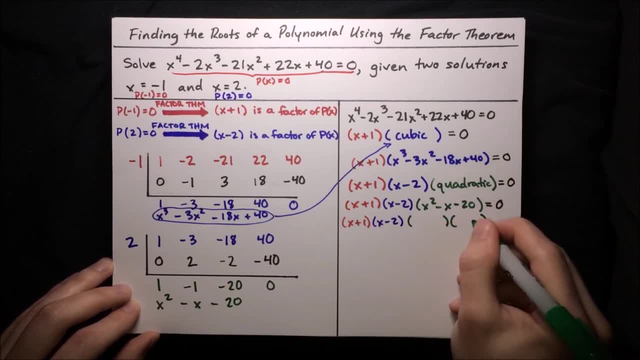 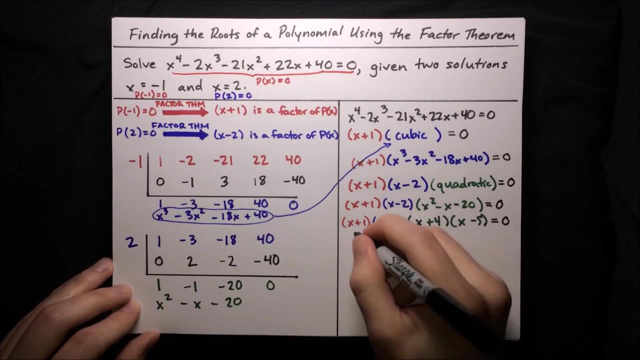 negative to sum to negative 1. So bigger one should be negative. How about negative 5 and then positive 4. Put our x's in Great, that works out. And then that has to equal zero. Great. So now we can use our zero product property to set each of these factors equal to zero. x plus 1 equals zero.